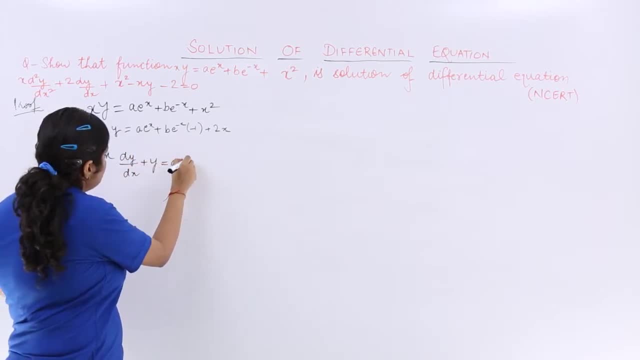 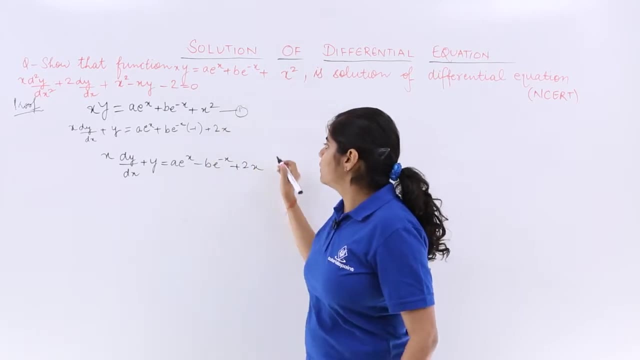 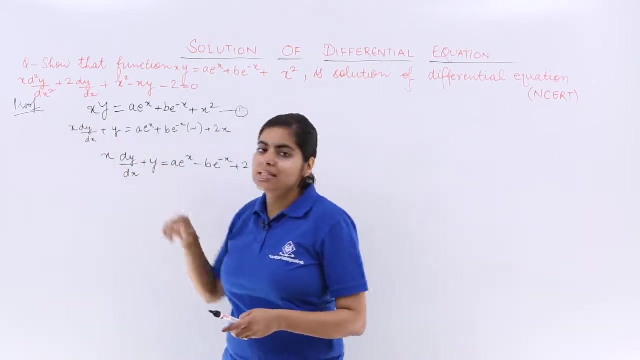 dy by dx plus y is equal to a. e raised to the power x minus b, e raised to the power minus x plus 2x. This is equation number 1.. This is equation number 2.. Now see what is needed. We need x. d2y by dx square, and so on means second order, derivative also, Okay, So let 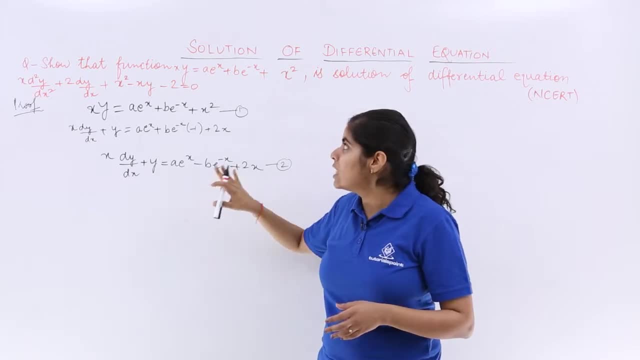 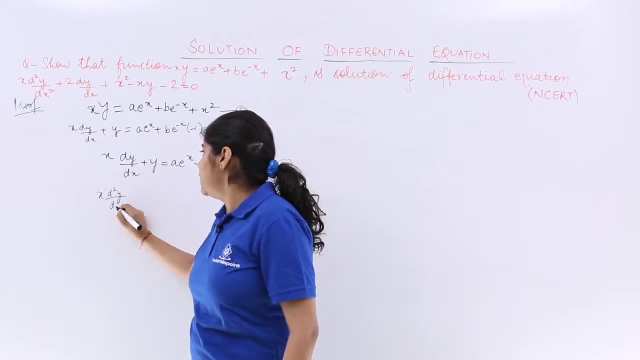 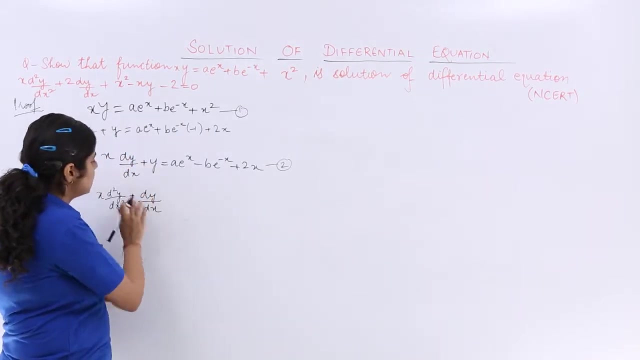 me find out the second order derivative from here only. So what is the second order derivative? So it should be x, as it is d2y by dx, square plus dy by dx, as it is, differentiation of x is 1 plus dy by dx, differentiation of y is 2.. So this is equation number 1.. So this: 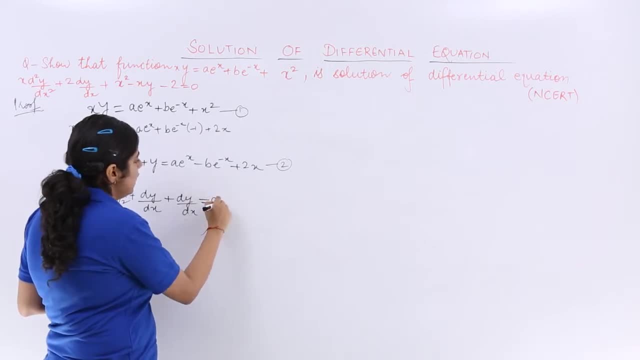 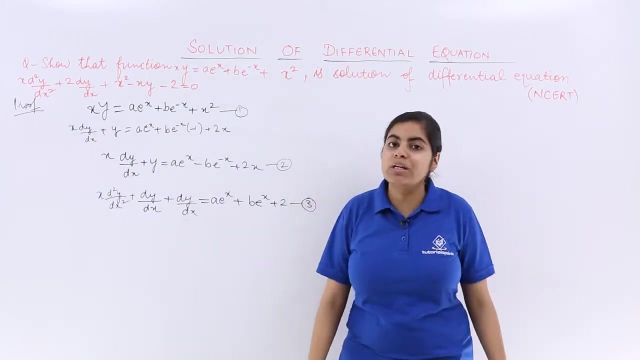 equation of y is dy by dx is equal to a, e raised to the power x as it is, Then here also the differentiation: again minus sign will come. So it is plus b, e raised to the power x plus 2, equation number 3.. Now you see, second order derivative has also been: 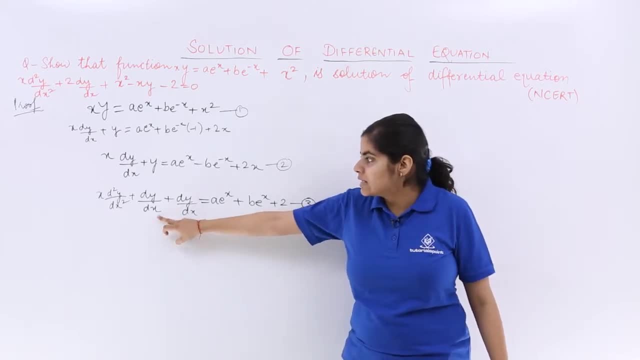 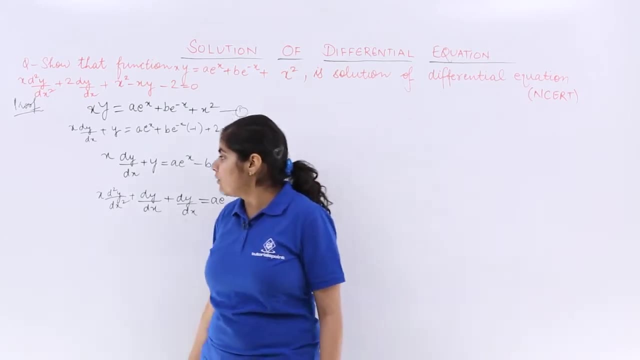 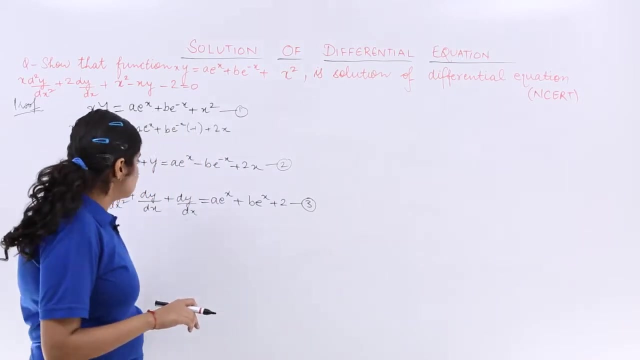 got in this step. Now this is what. This is: dy by dx plus dy by dx, which is 2 dy by dx. that I can change for sure in this step, So it should be 2 dy by dx. The other thing here, everything remains the same. So let me make one more equation, and or I can do the 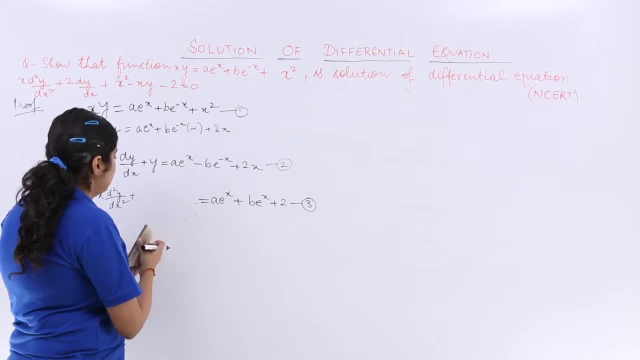 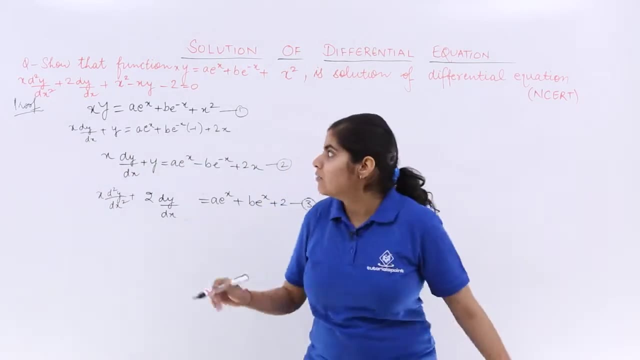 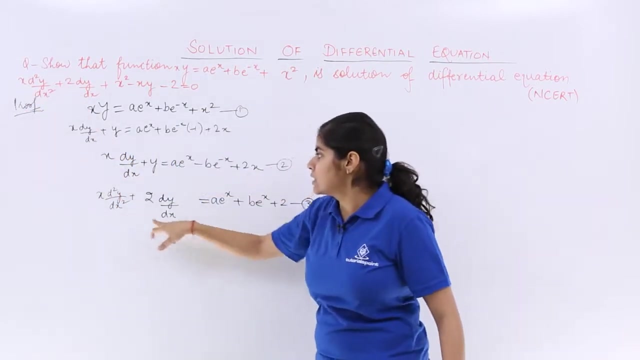 changes in this particular equation only. So this should be 2 dy by dx Right Now. what do we have to prove? We have to prove this particular fact wherein we have x, d2y by dx square plus 2 dy by dx. See, its value is already given, So what I can do is I can name this: 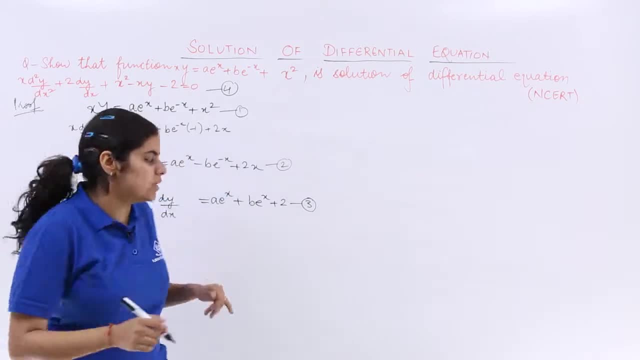 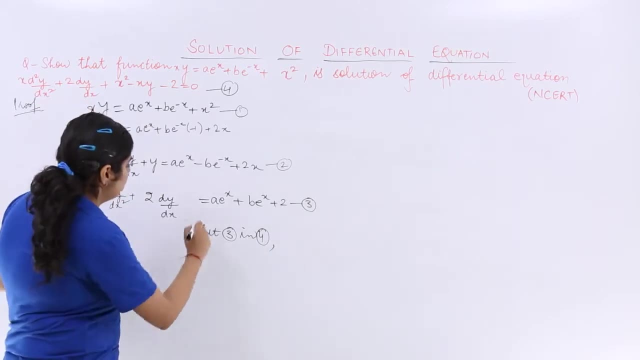 equation as equation number 4.. And I write: put my equation number 3 in 4.. So put 3 in 4.. So what do you have? The value is a, e raised to the power x plus b, e raised to the power x plus 2, and this should be minus.